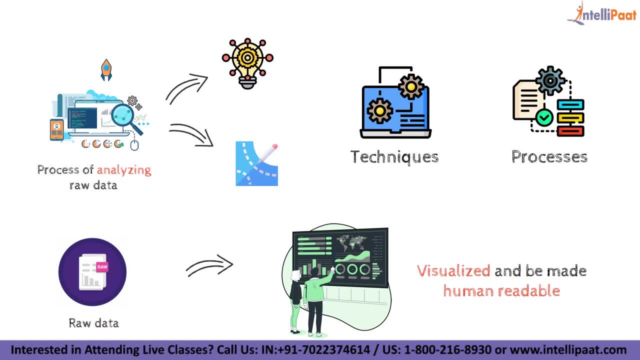 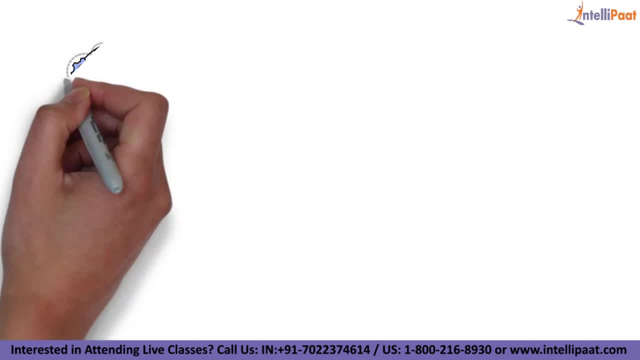 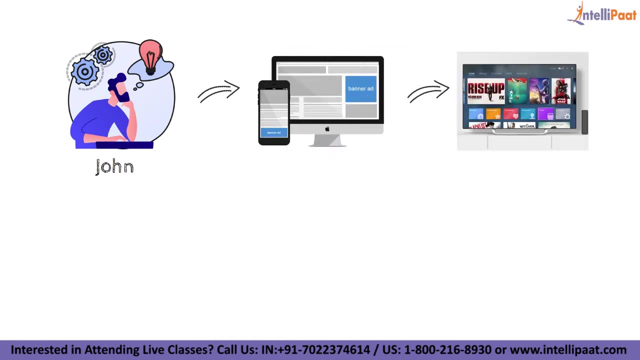 could be further visualized and be made human-readable To understand the definition in an even clear way. let's take a look at this example. John, who is a digital marketing professional, is running an online advertising campaign to promote a new smart television. John starts by targeting the group of people. 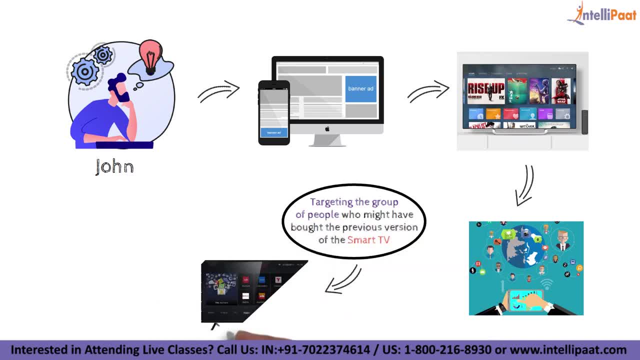 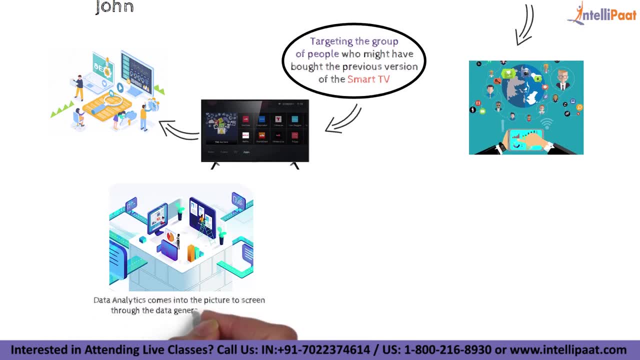 who might have bought the previous versions of the smart TV in question. As said campaign runs, data analytics comes into the picture through the data generated whenever people clicked on the public TV. Now, by inspecting the data about these users' interests and their buying patterns, you 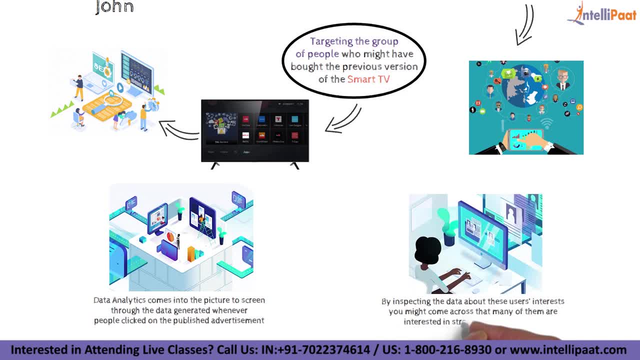 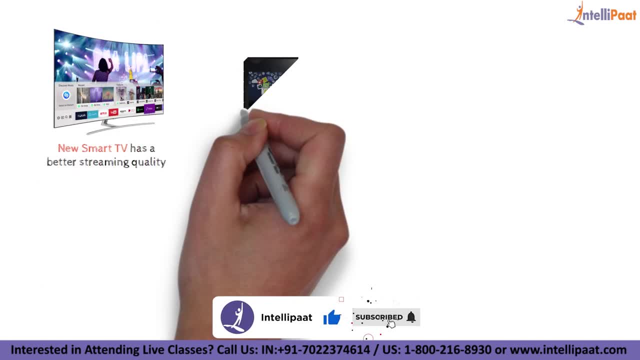 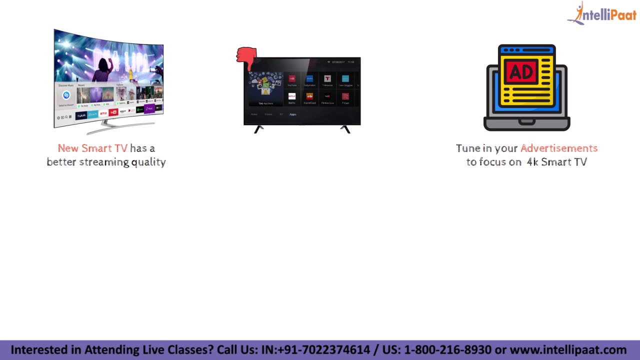 might come across that many of them are interested in streaming 4K UHD video. The reason behind this might be that the new smart TV has a better streaming quality than the previous versions. Using this information, you could tune in your advertisements to focus. 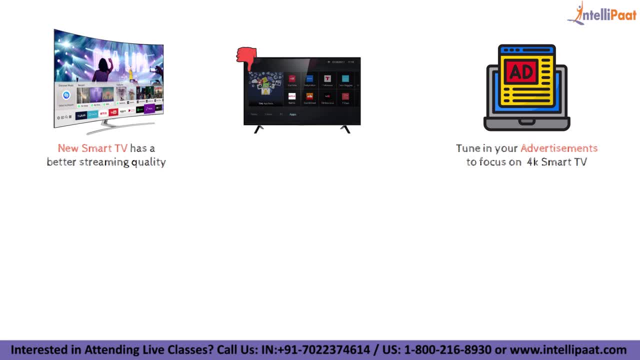 on users who bought the previous version of the smart TV. babanalongameraぎع ، Kollegejekimichaelisticknisand answer questions to any company that is interested in getting 4K streaming quality. This data can also be used to attract new customers. 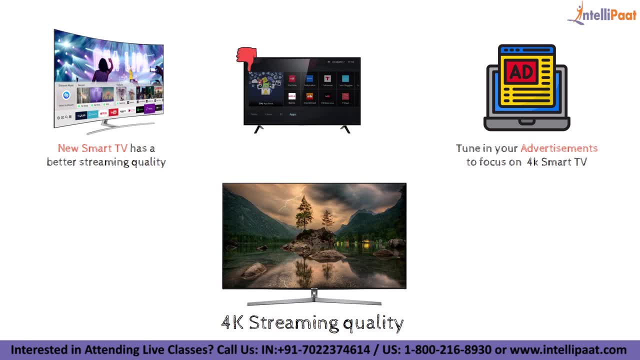 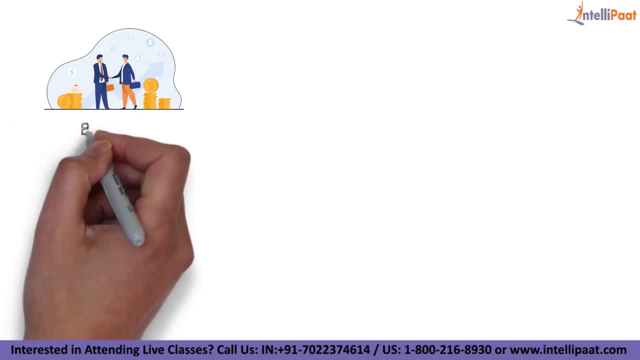 who did not go for the previous version of smart TV but are very interested in a better version of TV. Why is data analytics significant? Businesses use data analytics to optimize and grow by making big business decisions and finding more efficient ways of doing business. 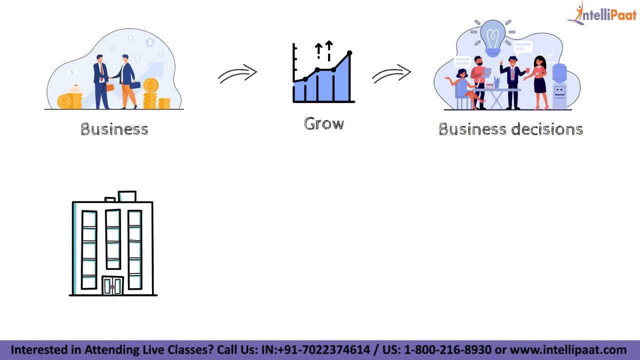 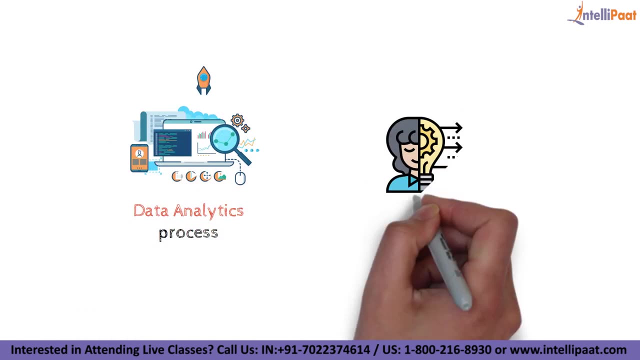 bourذا zad ton risk kolhPeže tera muslukiyo. This is basically what the business can do, entrada. The company can build new and better products, better understanding what the customers need. so how do data analytics work? the data analytics process has some components that can help a variety of 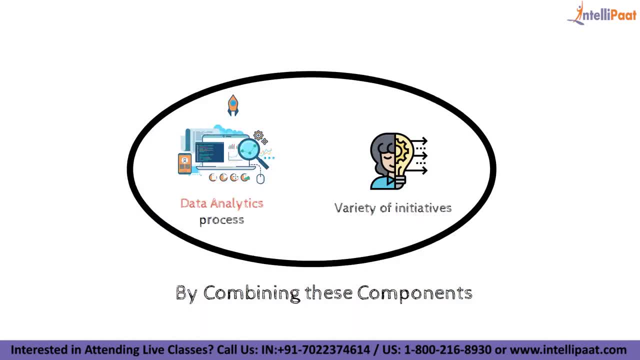 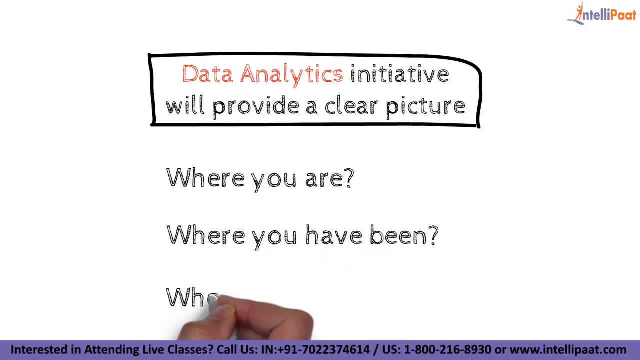 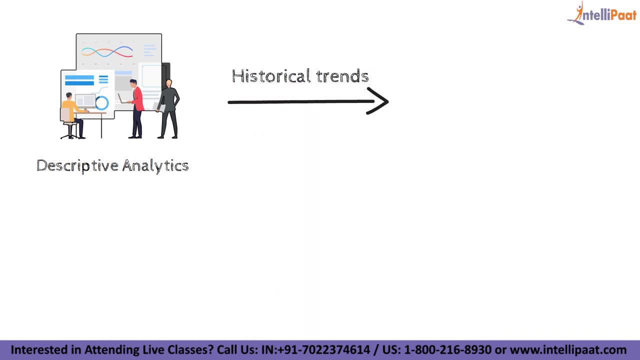 initiatives. by combining these components, a successful data analytics initiate will provide a clear picture of where you are, you have been and where you should go. generally. this process begins with the descriptive analysis. this is the process of describing historical trends in data. descriptive analytics aims to answer the question: what happened? this often involves 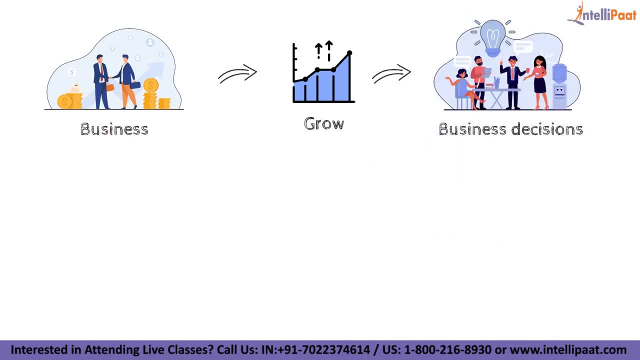 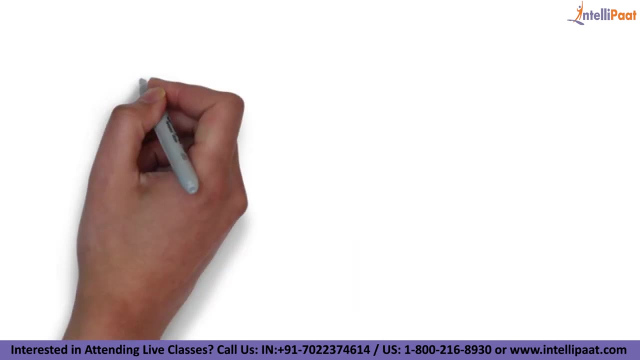 and grow. by making better business decisions and finding more efficient ways of doing business. The company can build new and better products with the buying patterns, for example, you patterns- and better understanding what the customers need. So how do data analytics work? The data analytics process has some components that can help a variety of initiatives. 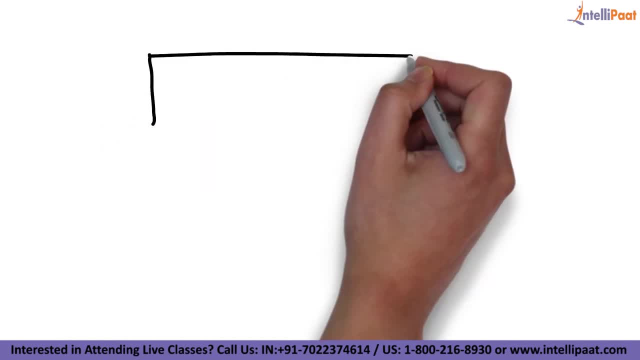 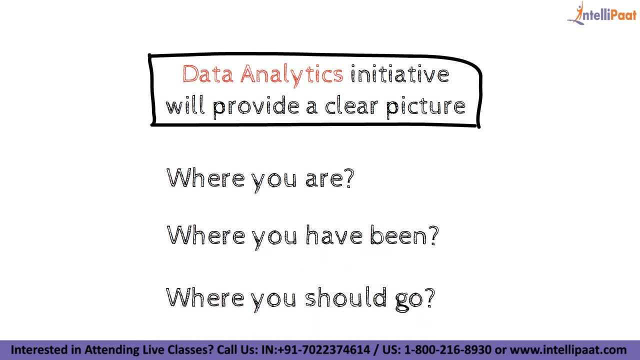 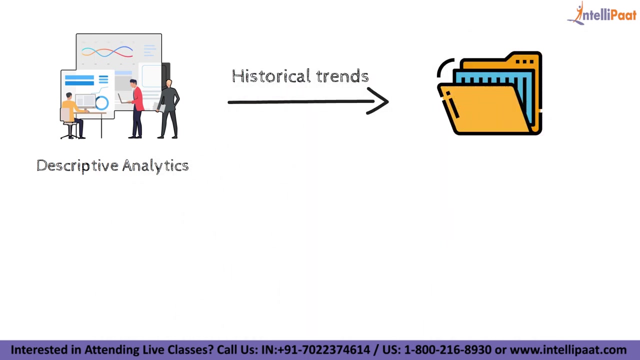 By combining these components, a successful data analytics initiate will provide a clear picture of where you are, where you have been and where you should go. Generally, this process begins with descriptive analysis. This is the process of describing historical trends in data. 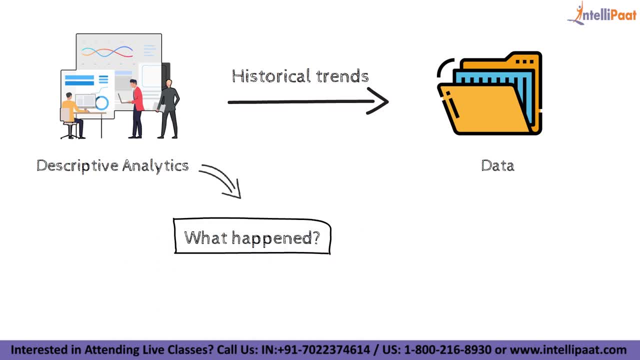 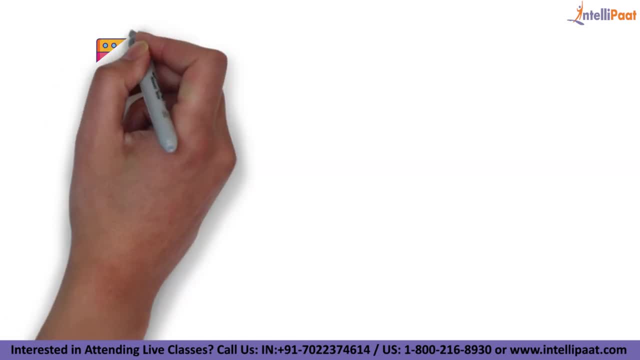 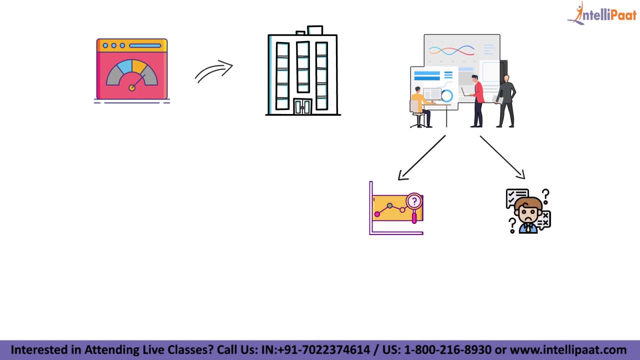 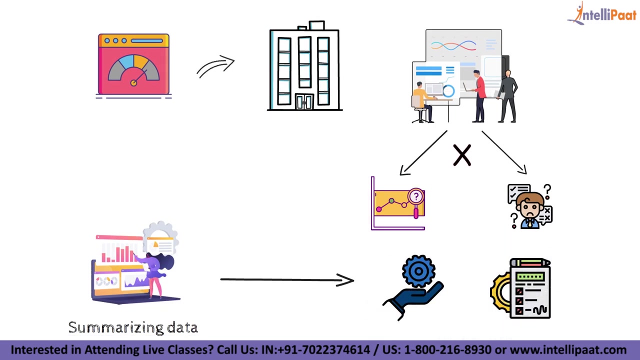 Descriptive analytics aims to answer the question: what happened? This often involves measuring traditional indicators such as return on investment. The indicators used will be different for each industry. Descriptive analytics does not make predictions or directly inform decisions. It focuses on summarizing data in a meaningful and descriptive way. 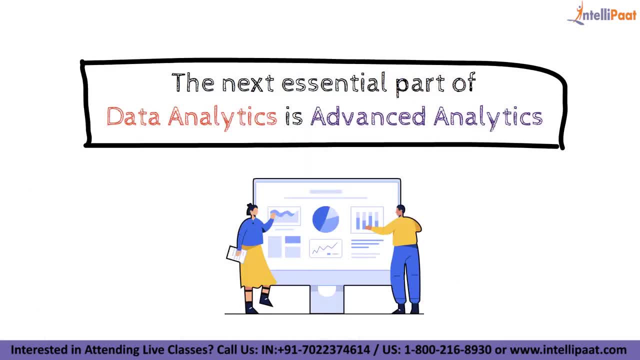 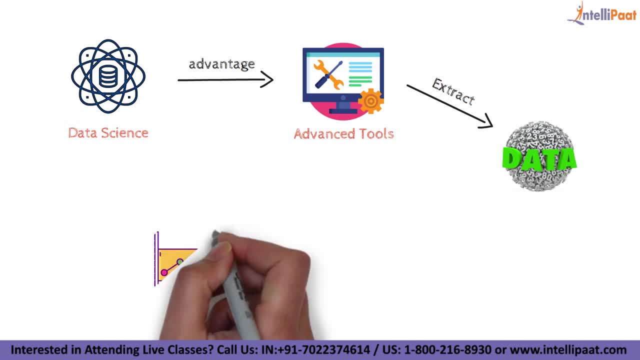 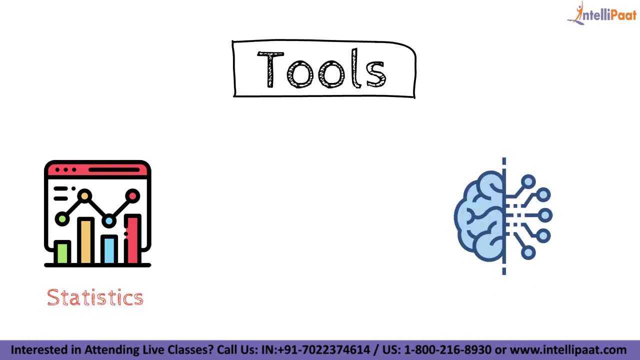 The next essential part of the data analytics process is data analysis. The next essential part of data analytics is advanced analytics. This part of data science takes advantage of advanced tools to extract data, make predictions and discover trends. These tools include classical statistics as well as machine learning. 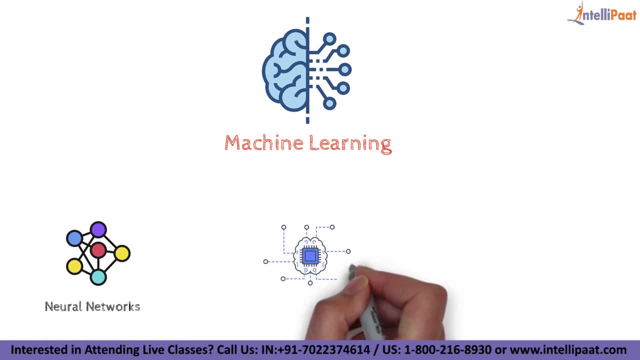 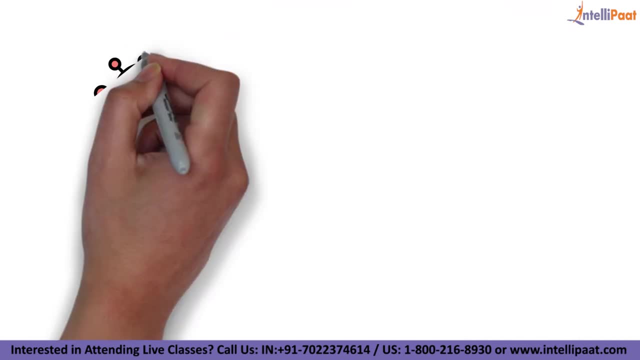 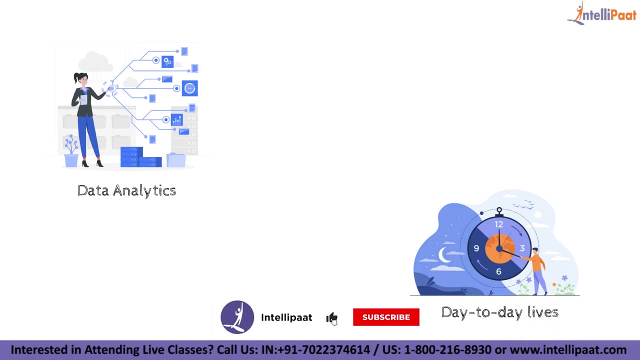 Machine learning. techs such as neural networks, natural language processing, sentiment analysis and more enable advanced analytics. This information provides new insight from data. Advanced analytics addresses the what-if question. Data analytics affects every aspect of our day-to-day lives. You may not even realize it, but you probably use data analytics almost every day. 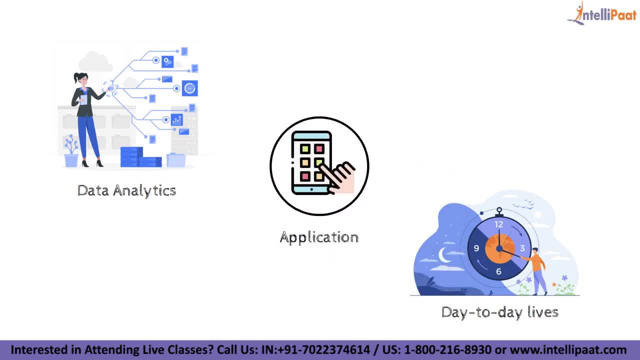 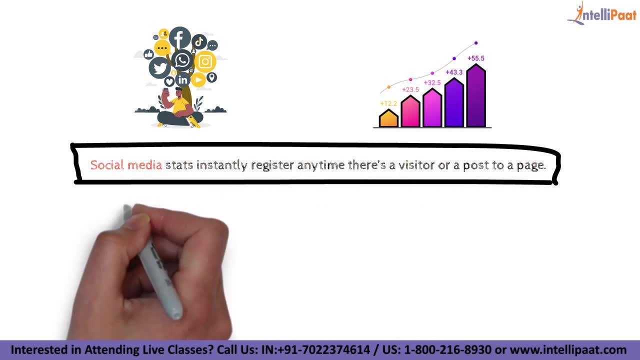 Here are some of the everyday applications of data analytics. Social media stats instantly register any time there's a visitor or a post to a page. Cell phone bills can pull up months of data. This is the first step. Data analytics is the first step of calling data to show you patterns of usage. 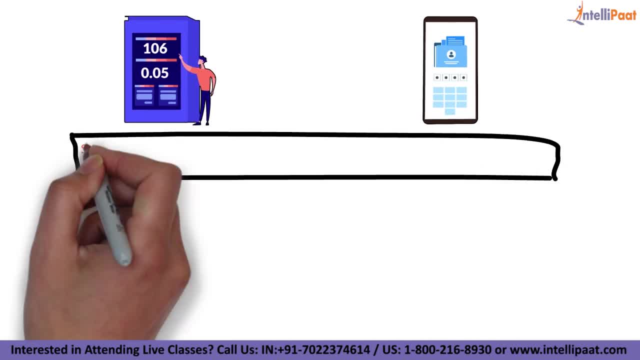 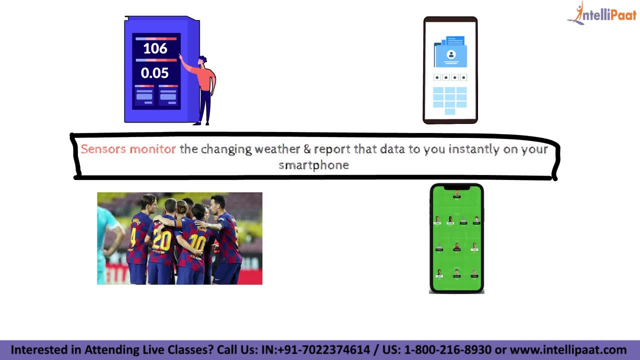 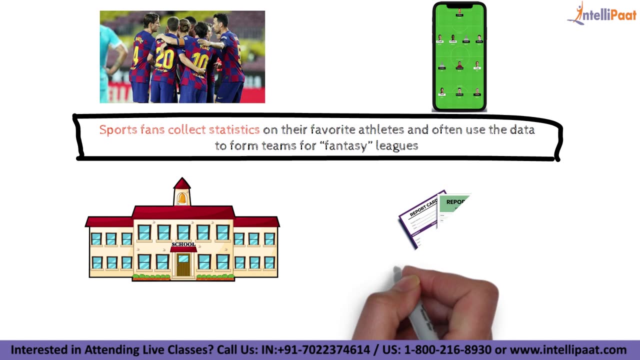 Sensors monitor the changing weather and report the data to you instantly on your smartphone. Sports fans collect statistics on their favorite athletes and often use the data to form the term of fantasy leagues. Schools across the nation are involved in high-stakes testing that generates voluminous 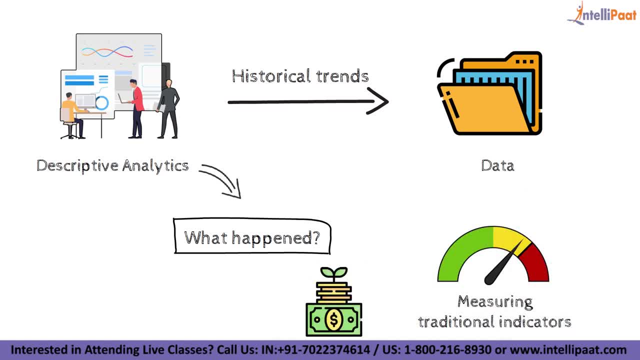 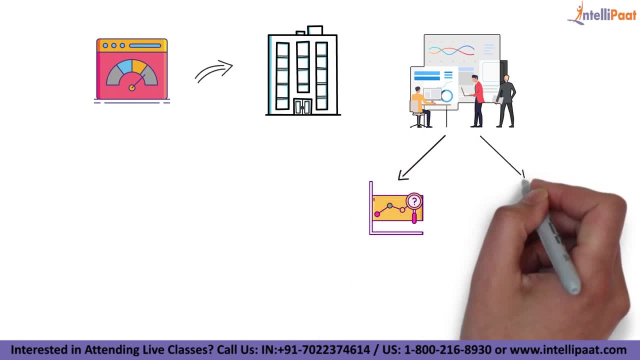 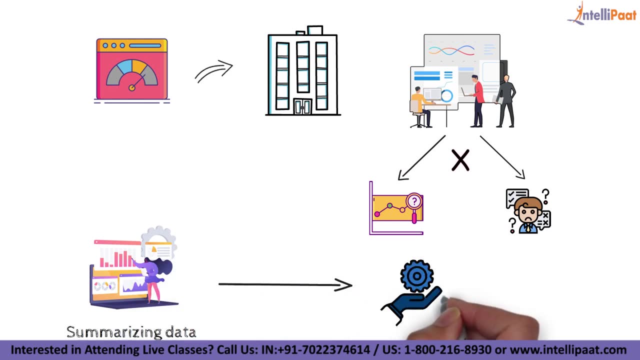 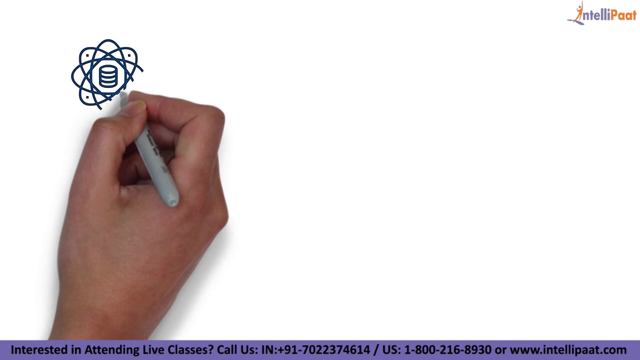 measuring traditional indicators such as return on investment. the indicators used will be different for each industry. descriptive analytics does not make predictions or directly informed decisions. it focuses on summarizing data in a meaningful and descriptive way. the next essential part of data analytics is advanced analytics. this part of data science takes advantage of advanced tools to extract. 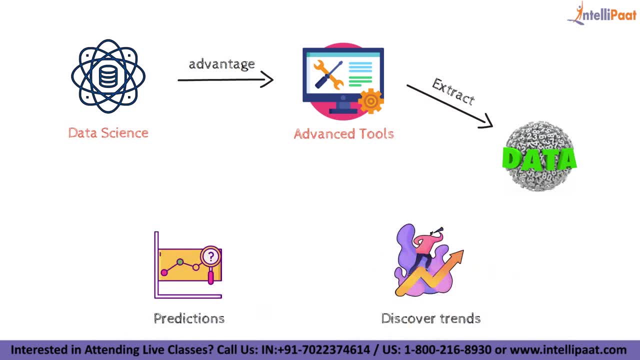 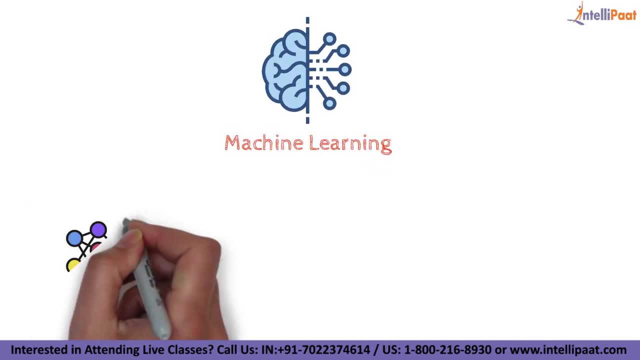 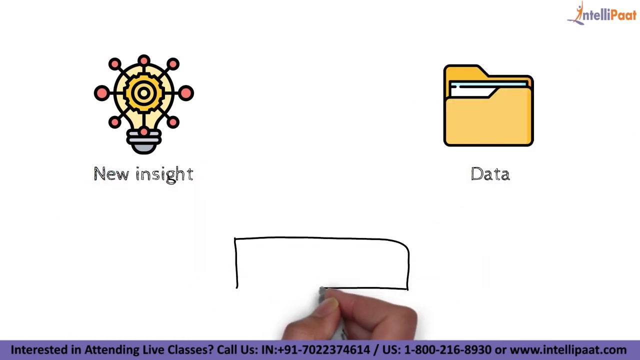 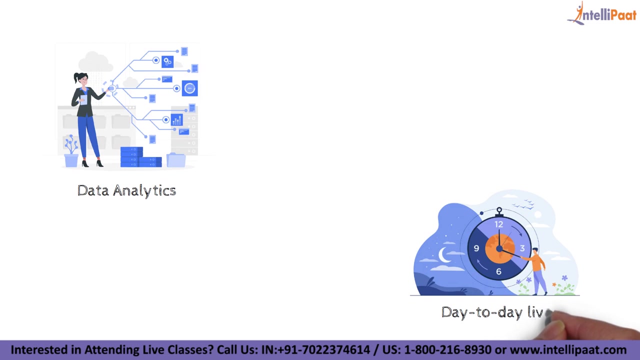 data, make predictions and discover trends. these tools include classical statistics as well as machine learning. machine learning, texts such as neural networks, natural language processing, sentiment analysis and more enable advanced analytics. this information provides new insight from data advanced analytics addresses. what if the question data analytics affects every aspect of our day-to-day lives? 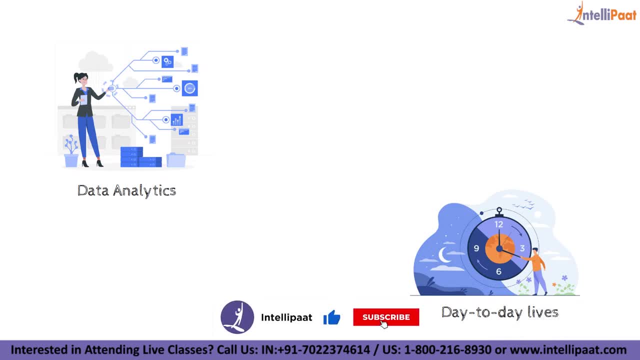 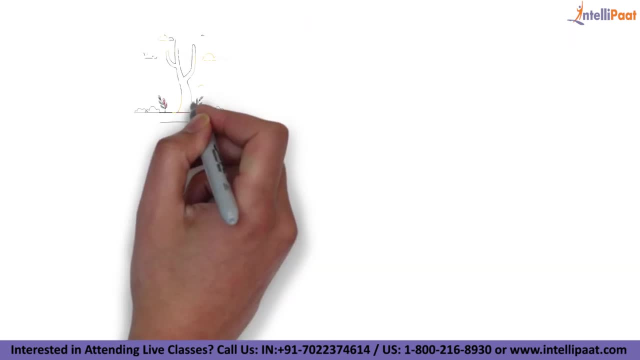 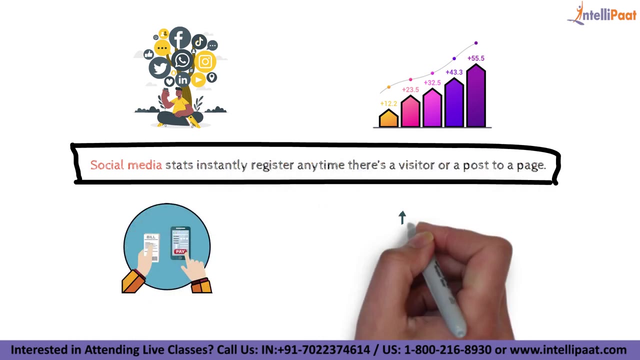 you may not even realize it, but you probably use data analytics almost every day. here are some of the everyday applications of data analytics: social media stats instantly register anytime there's a visitor or a post to a page. cell phone bills can pull up the list of what i'm asked about. for what is the thing that you want to? 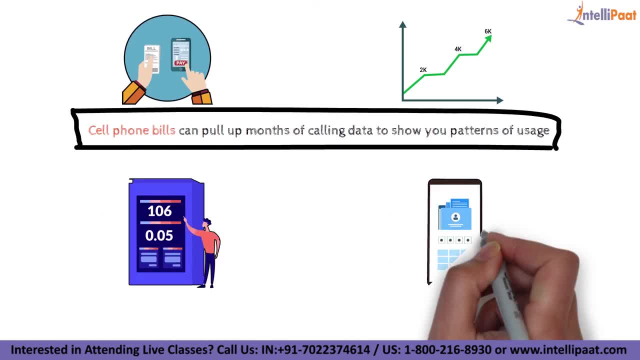 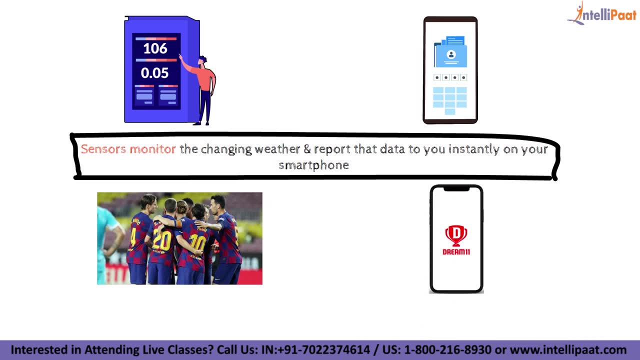 do now and when did i pick this up, how it works and how to use it. so data analytics requires a lot of expertise to know how to gather data in the right way. data analytics will deliver an awesome image in a short time. data analytics can help you track whose phone is ringing or what is the time. 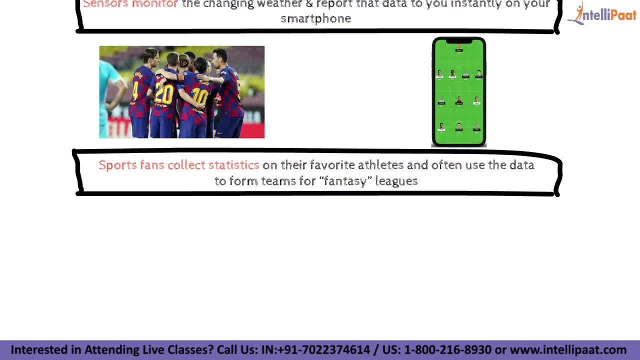 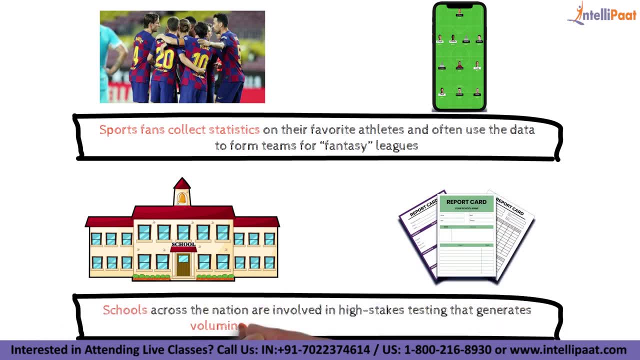 last minute. i have been working at the same computer and i've been working for months on the same computer. i was watching sports media while i was editing my peux, but now i've already know how to use data analytics in mydata. mydata is a very easy way to output data analytics that is um. 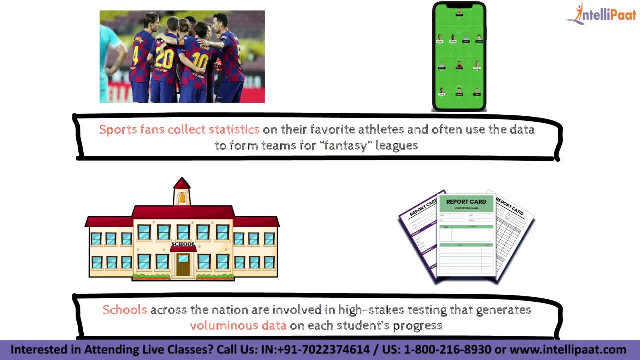 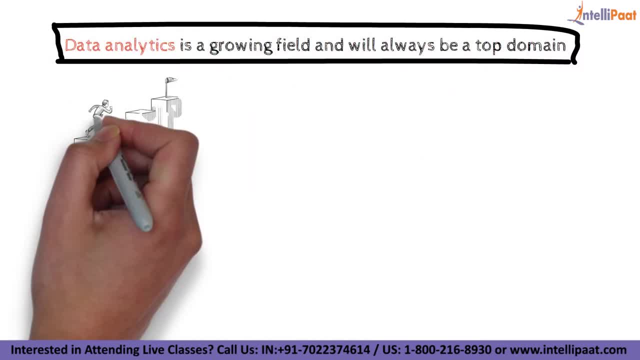 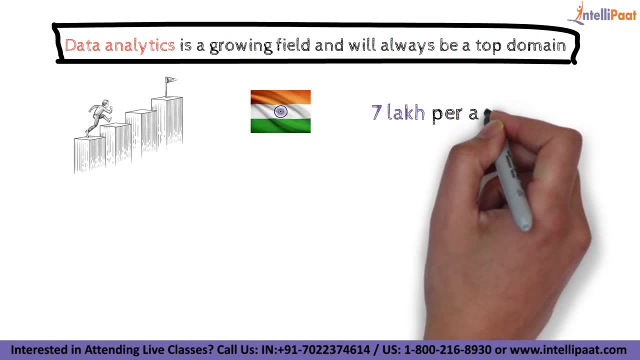 easy and easy to use. data analytics shows the time that data analytics take. Users then utilize data generated from extensive reports to drive their instruction. Data analytics is a growing field and will always be a top domain to get into. The average salary of a data analyst in India is 7 LPA and in the US it's $70,000.. 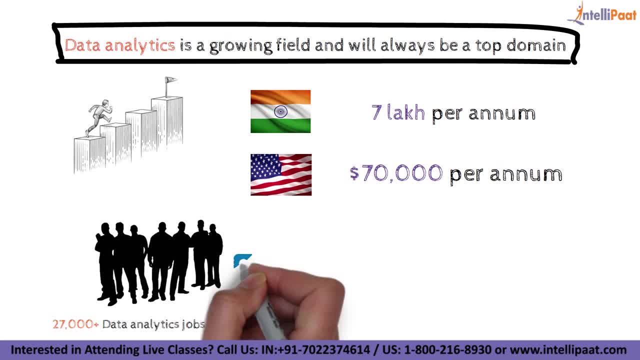 There are 27,000 plus data analytics jobs available only on LinkedIn and there are very few skilled professionals to fill that gap. That's all about data analytics.